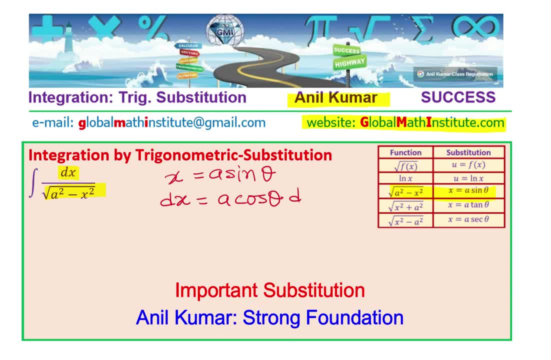 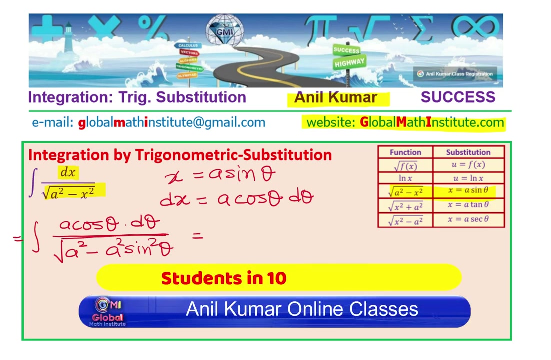 Correct. Using this substitution we get this integral. So instead of dx we will write a cos, theta, d theta, And the denominator will be square root of a square, minus a square sine square theta. Right Now in the denominator we could factor out a square. 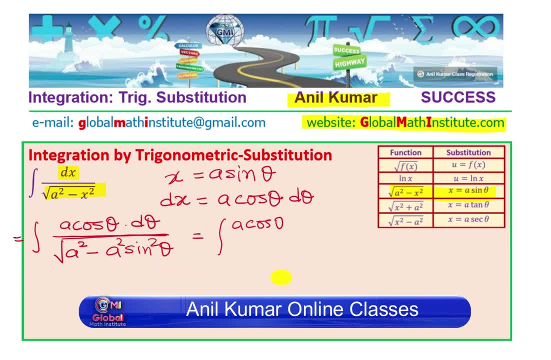 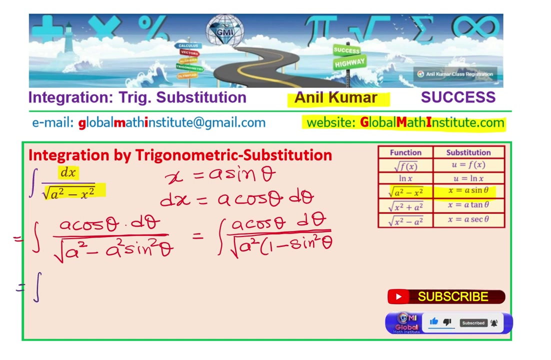 So in the numerator we have a cos theta And in the denominator we have a cos theta d theta. Factoring a square we get 1 minus sine square theta square root. So we can further reduce this to a cos theta d theta. 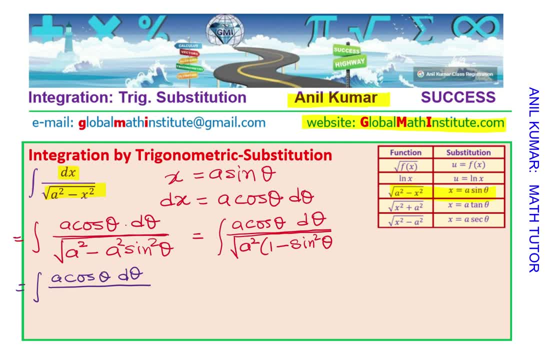 And in the denominator we have a cos theta d theta. a square comes outside, So we get a, And 1 minus sine square theta is cos square theta Right. So we have square root of cos square theta. This can be written as integral of a cos theta over a cos theta. 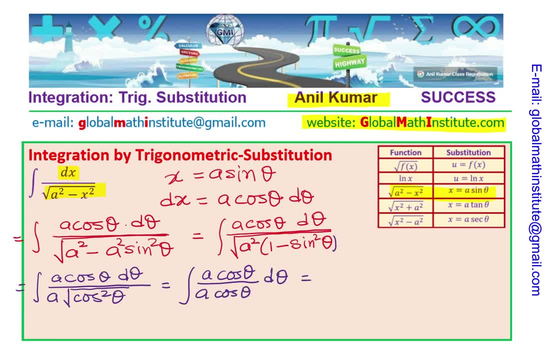 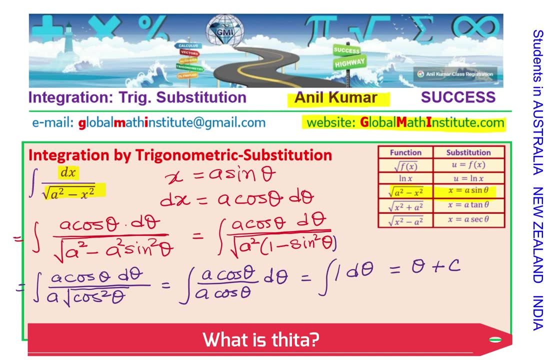 Do you see d theta? So that is integral of 1 d theta, Or the solution will be theta plus c. Make sense. So that is the solution. Now, what is theta? So when you write x equals to a sine theta. 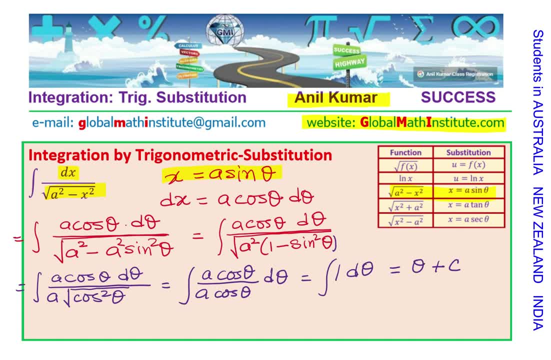 then theta is x over a, sine, inverse of that, Correct. So let us do that part also. So we know that sine theta is equal to x over a. That gives you theta as equal to sine. So we know that theta is equal to sine, inverse of x over a.